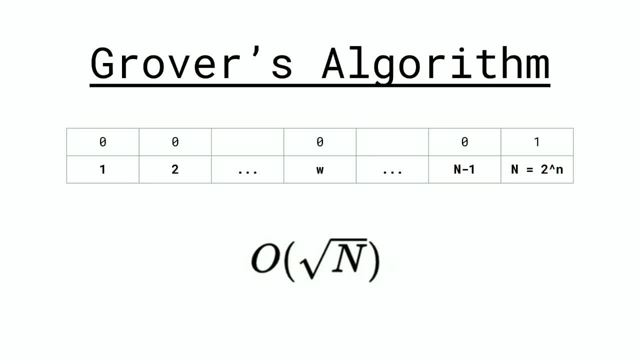 which is a very big speedup from classical computers. If we were to imagine n would be a million, then a classical computer could solve it in a million steps, while Grover's Algorithm could solve it in a thousand steps, which is, as you can see, a very big speedup. 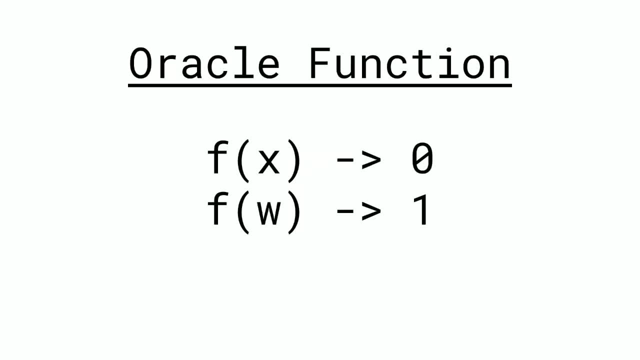 Just like the Deutz-Joseph problem. what we're going to do is have an oracle function which we're going to put qubits and superposition through. Now, what this oracle function does for an unstructured search is very simple. 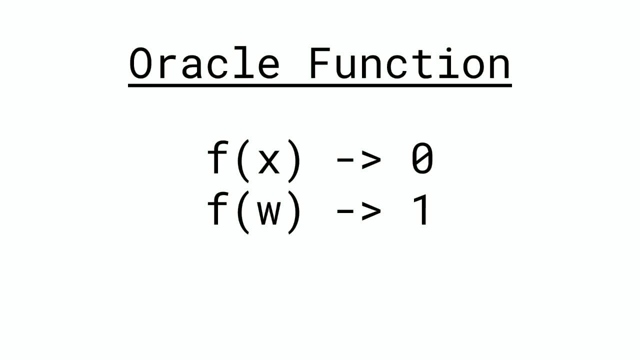 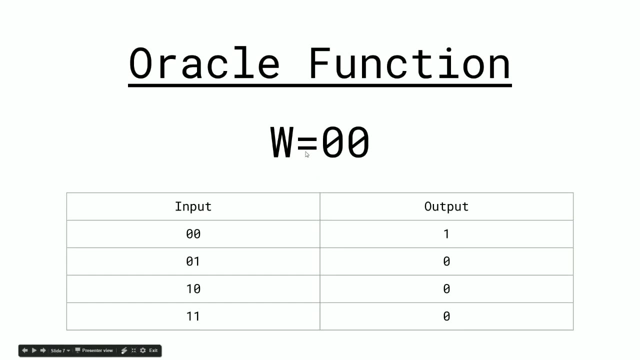 It outputs 0 if the input is x- anything we're not looking for- It outputs 1 if the input is W, the value we are looking for. So, for example, if we were to be looking for, W equals 0, 0,. 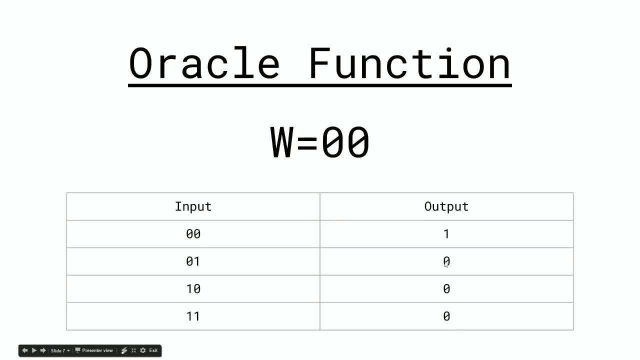 the oracle function would output 1 for 0,, 0, and 0 for every other value. Now, by using the amplitude and by multiplying at the amplitude that this oracle function creates, we're able to output what the correct W we're looking for is. 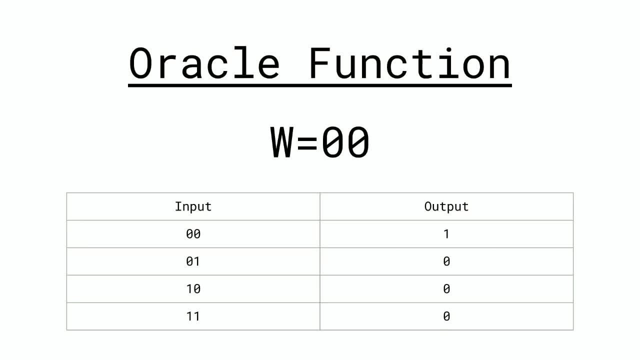 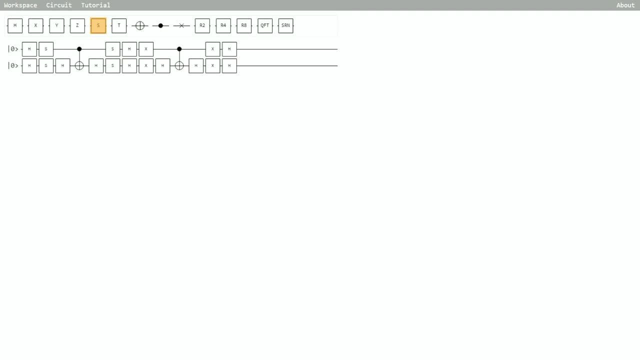 So let's look at an implementation of this on the simulator. So here we have a simple circuit implementation for solving Grover's Algorithm, And what this is doing is it's searching for the input 0,, 0,, which is what we were examining in the last slide. 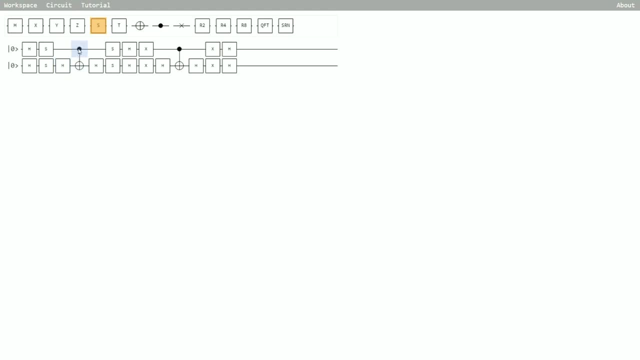 So where the 0, 0 is encoded is in these two oracle functions right here, which we have to invoke twice because n is equal to 4. in this case It'll run times, the square root over n, which is equal to 2.. 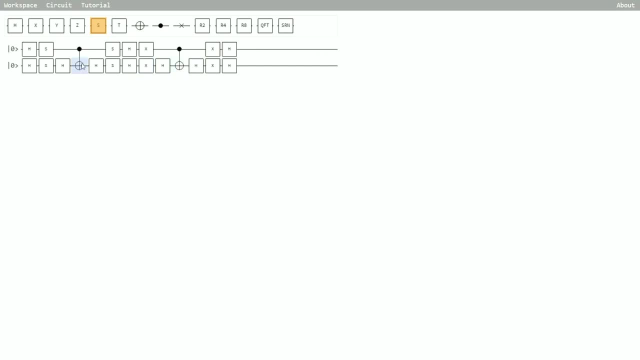 So we have to invoke the oracle twice Now. just like the Deutsch-Jozza Algorithm, Grover's Algorithm has three different steps that it does. The first is to put the qubits through Hadamard gates, to put them in superposition. 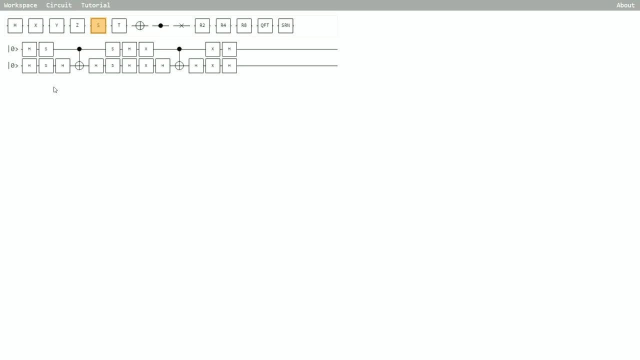 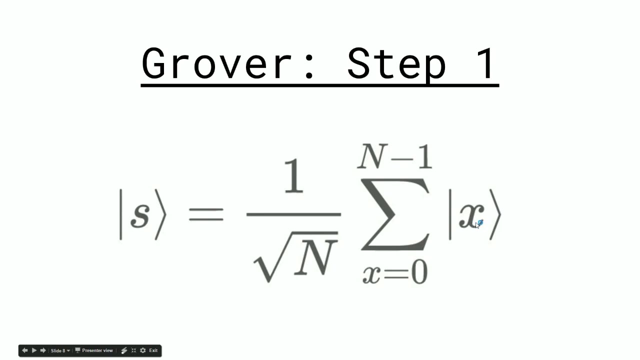 which is similar to what we've been doing in the other video tutorials, And this can be represented by this equation, which essentially says that it's putting the qubits into every different possible input, for x being represented here. Now, what this does is this: makes the qubits 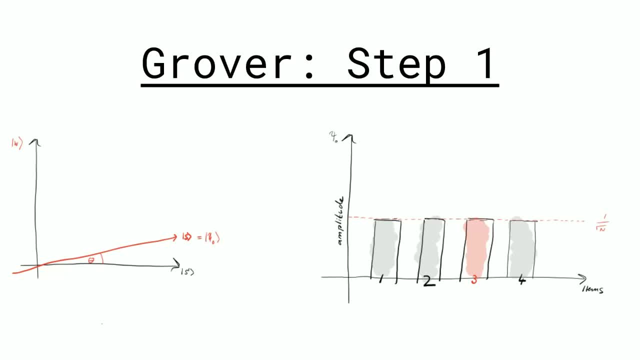 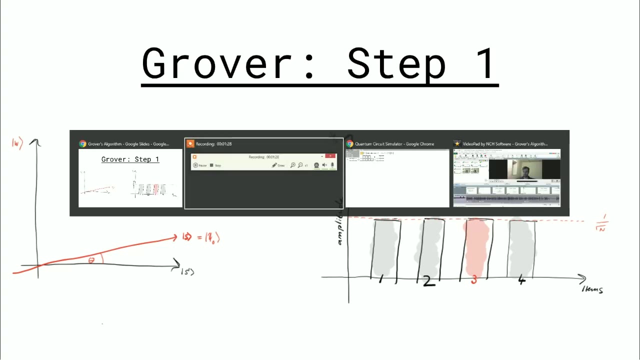 have a uniform amount of amplitude, So the expectation value of any of the different possible inputs is going to be equal to 25% in this case. Now, when we perform the second step of Grover's Algorithm, which is putting it through the oracle function, 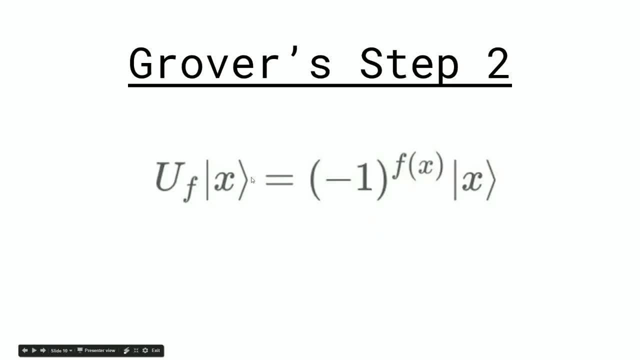 what ends up happening is we can see from here- remember this is very similar to Deutsch's Algorithm. if the oracle function evaluates to 1, this means that its eigenvalue is going to be negative 1.. But if the input is any item that we're not looking for on the list, 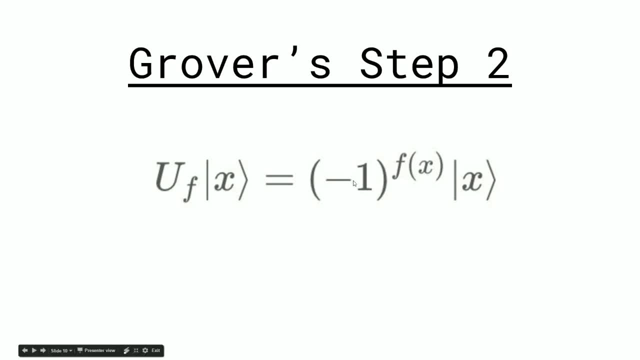 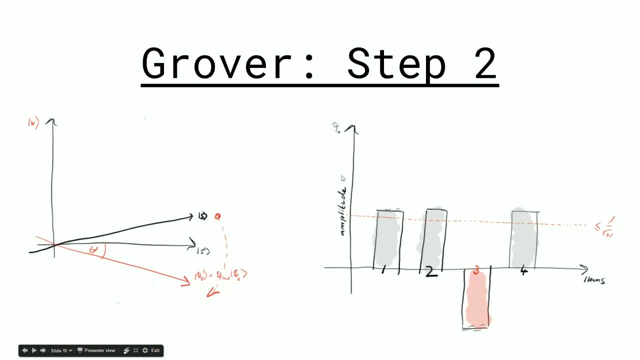 then the eigenvalue is going to be equal to 1.. Now what this has the effect of doing is flipping the amplitude of just the item that we're looking for, Because the eigenvalue is now going to be negative 1. And it flips only the input that we're looking for. 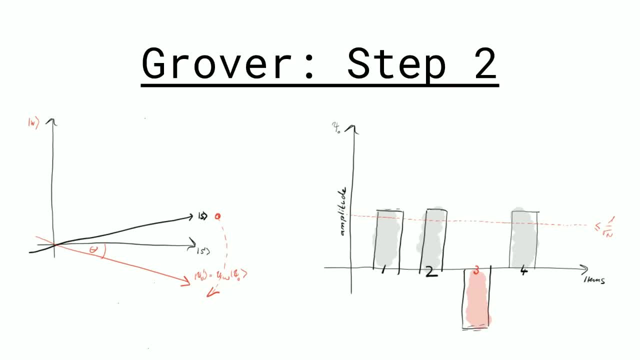 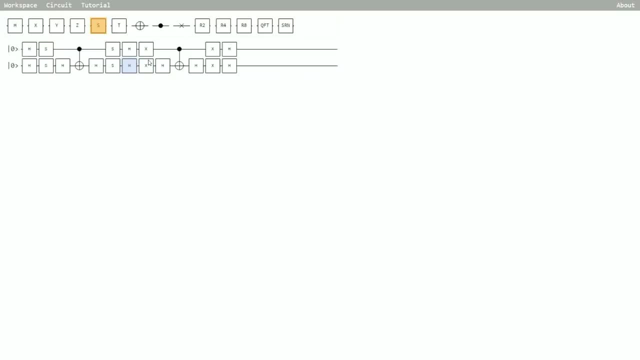 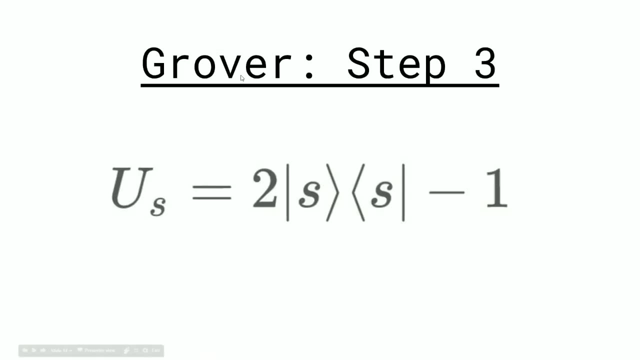 and leaves the other how it is. So when we now perform step 3 of the algorithm, which is putting the Hadamard gates again on the qubits after putting them through the oracle function, what we get is this: applying a state change to the qubits. 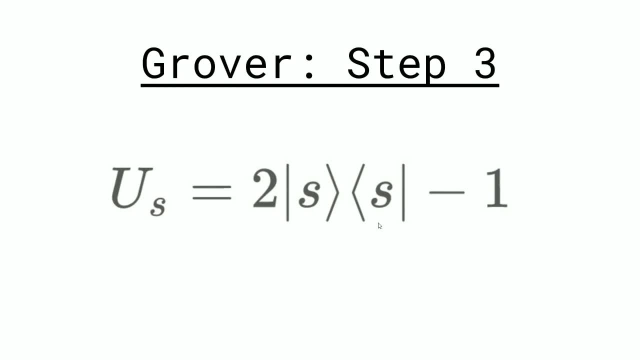 which once again reflects the input that we're looking for around the x value again, which then gives us the probability or the amplitude of the input that we're looking for at time. t plus 1, once we apply the oracle matrix on it and the Hadamard gate. 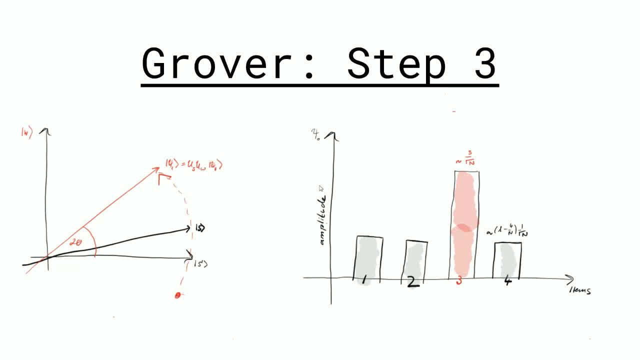 Again on it. And what this does is it flips the input value we're looking for, but amplifies it and increases it. So now the probability of us of the expectation value is going to go up And when we measure these inputs we're going to have a much higher chance of finding it. 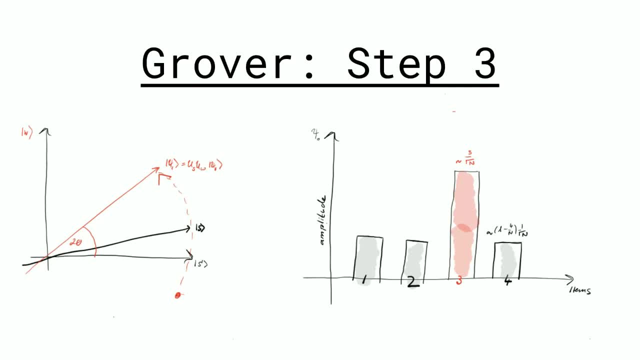 So what we do is we then repeat step 2 and 3. On each other until the amplitude here reaches close to w, And when we take a measurement, then there's going to be a very high probability of the results that we got. 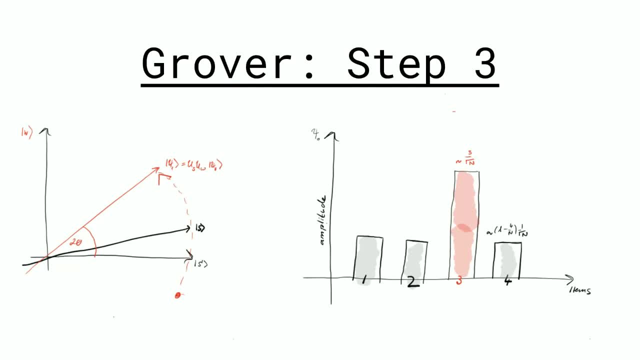 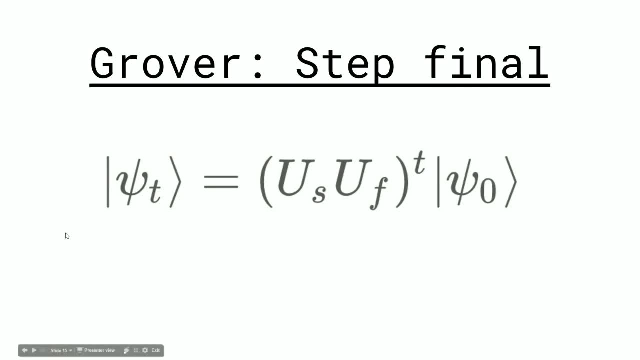 the observables that we saw from the qubits are going to be the item that we're looking for, And here we can see. the final step then is after we perform steps 2 and 3 at t amount of times we're going to get the amplitude in time t. 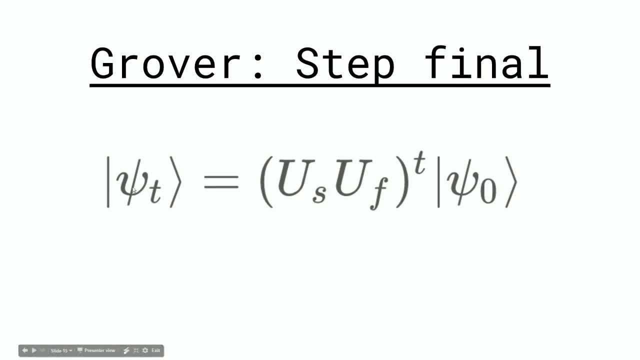 Now, why is the runtime square root of n? This is now kind of easy to see, because the amplitude of the item we're looking for is going to increase linearly. But because we're looking at probabilities, we have to, or we're looking at amplitudes. 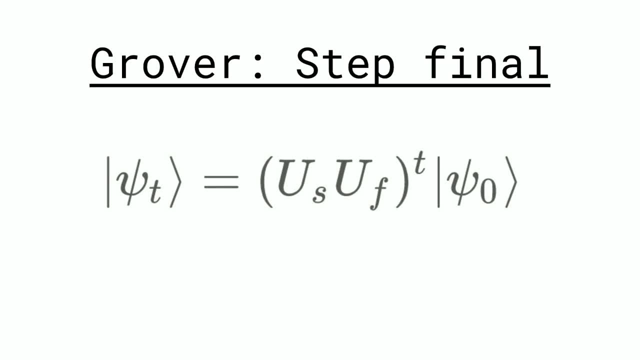 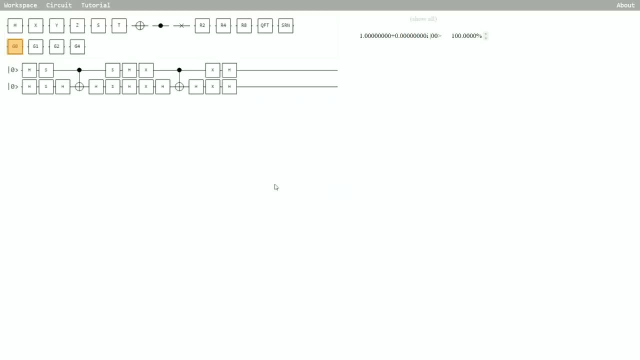 we have to take the square root of those, those amplitudes, in order to get the desired we're looking for, which is how we get a runtime of square root of n. So now let's actually run this circuit and find out what happens. 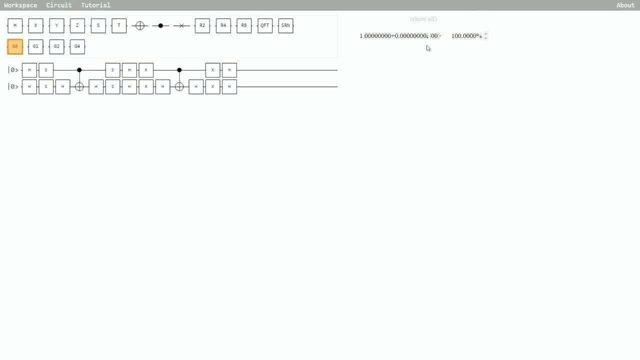 So, just like we were talking about, when we run this only once, by invoking the oracle function two times, we find that this algorithm finds the value we're looking for: 0, 0, with 100% certainty, with a 100% expectation value. 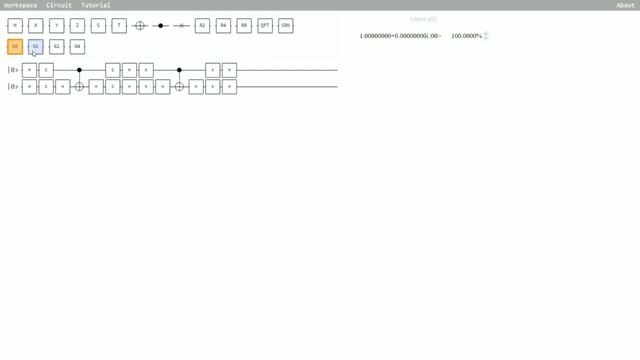 Now, if we were to encode a different value that we're looking for, say this one which we're now looking for, 0, 1, if we run this one again, we see that it also finds the value we're looking for.